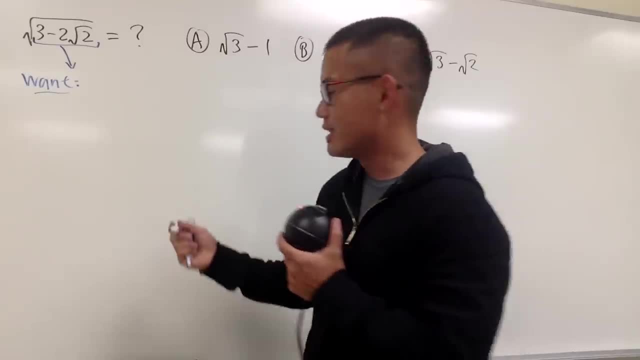 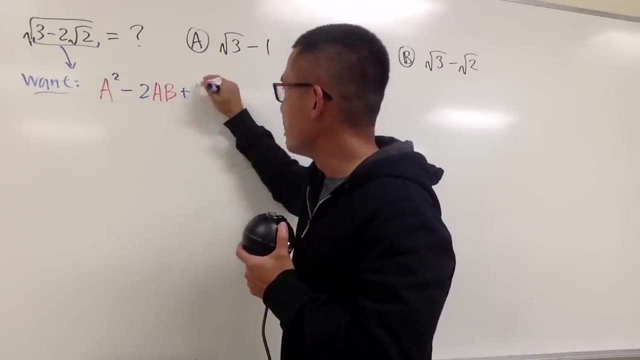 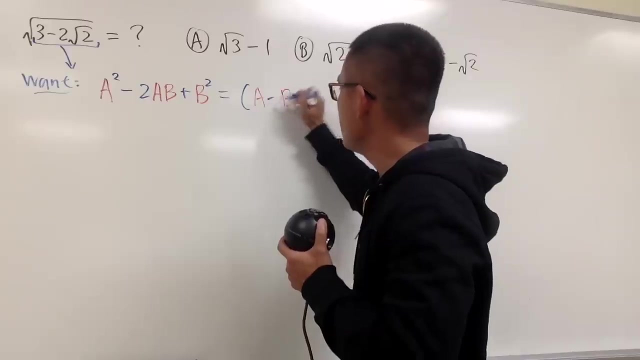 And since we have the minus right here, let me write down this for you guys. We know, when we have a square minus 2ab and then plus b square, this right here is a perfect square, isn't it? Which is going to be a minus b and then square right. 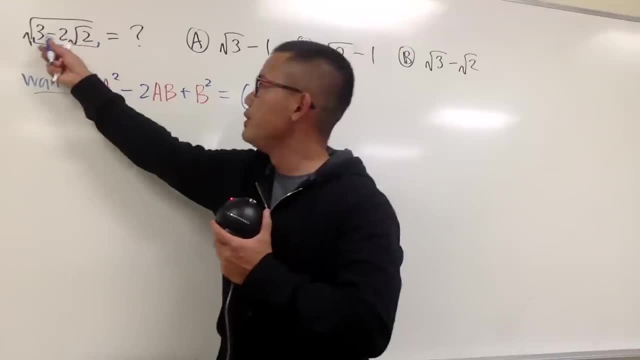 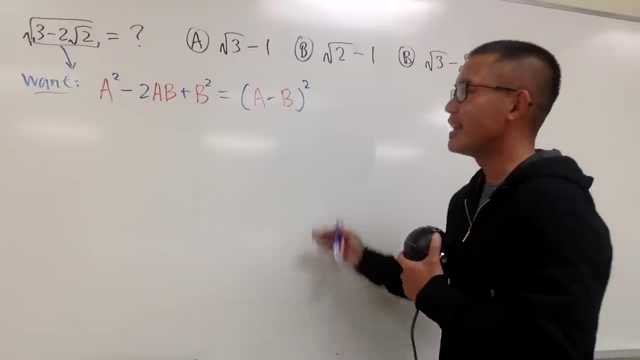 And, with this being said, can I make 3 minus 2, square root of 2 into this form? Because if I could do that, then I can complete a square like this And then I can cancel this square and that square root on the outside isn't it? 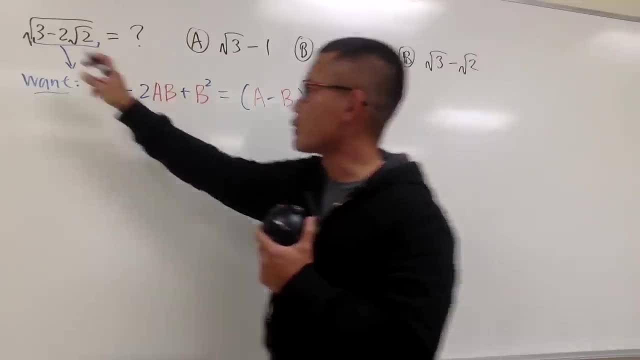 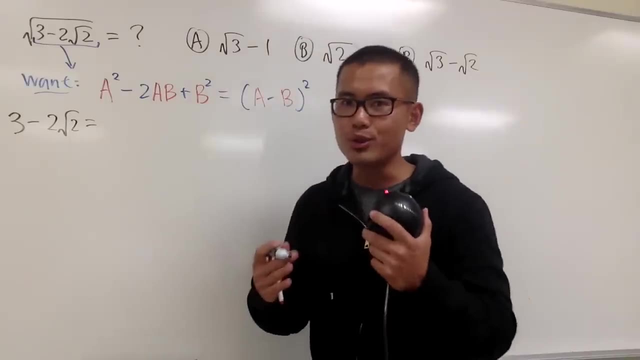 And that would be so wonderful. right, And now let me just write this down: right, here We have the 3, right here, and then minus 2, square root of 2, right, And now we are just going to try to mix and match, alright. 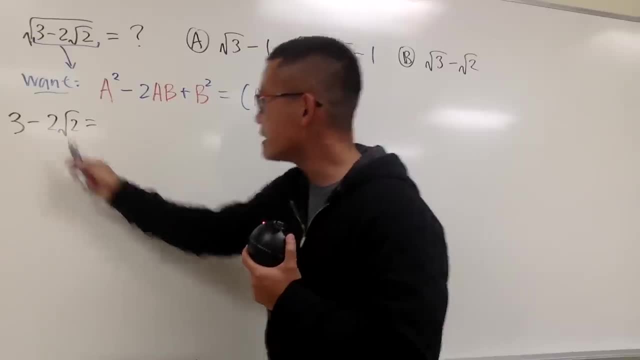 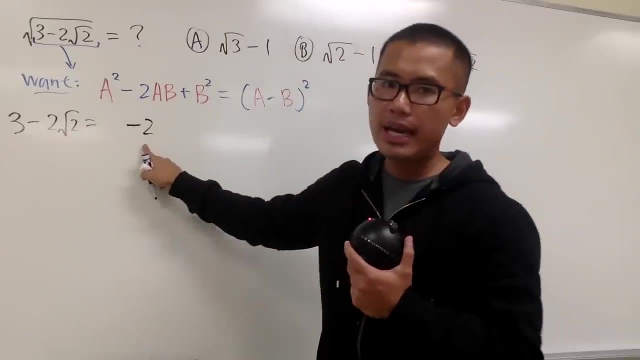 First of all, I have this minus 2.. This suggests me it's right here, isn't it? So let me put this down right here. We have the minus 2 from here, And we have to attach the square root of 2 after that. 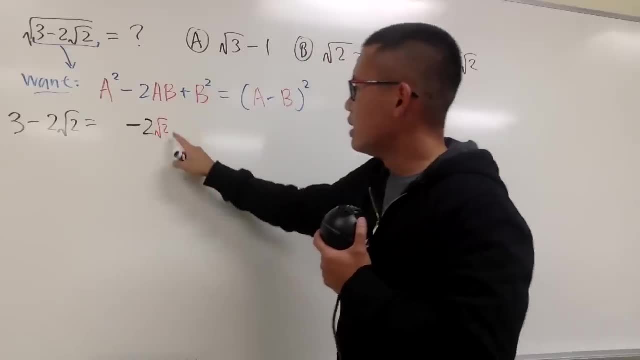 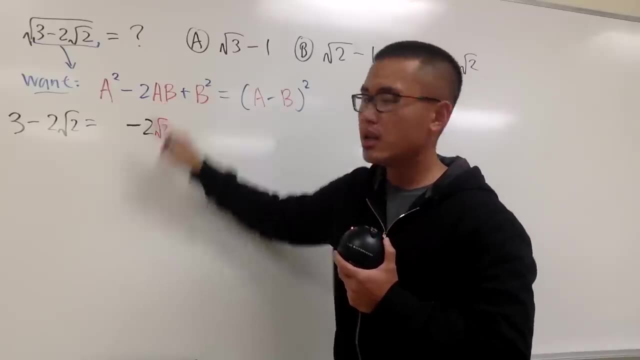 So let me just put down the square root of 2 right here And this square root of 2 in red. it could be either the a or b right. Well, suppose this is for a. then I will have to put the square root of 2 right here, underneath this square right. 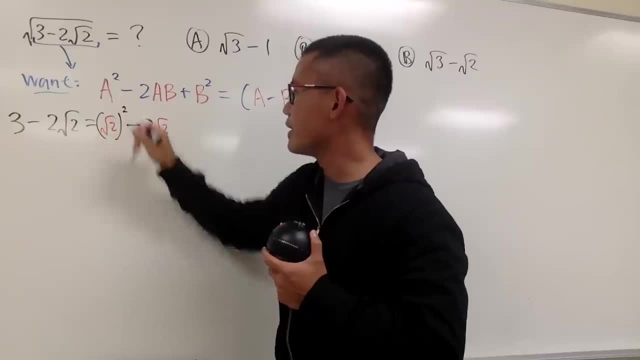 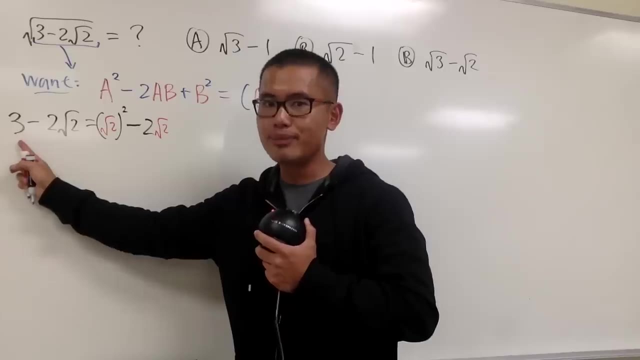 So I have square root of 2 like this and then I have to square that. But what's this? Square root of 2 squared is just a regular 2.. If you look back here, this is what We have: 3.. 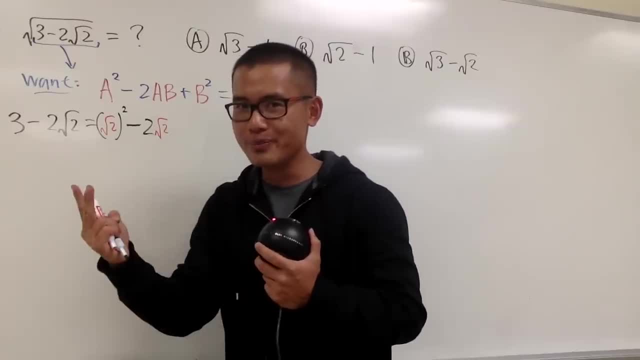 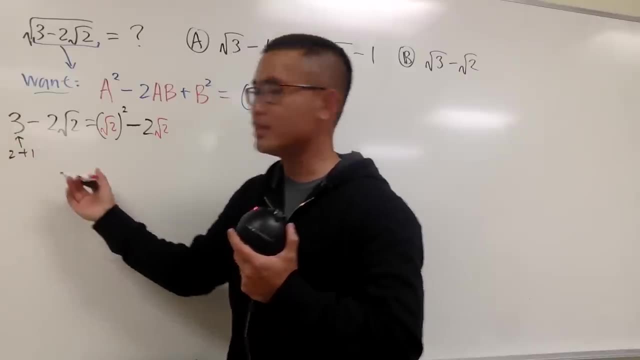 Well, 3 is certainly 2., But then you just have to add 1 to that right. So if you look at 3 as 2 plus 1, then we can make a lot of good things happen. First of all, this 2 is right here. 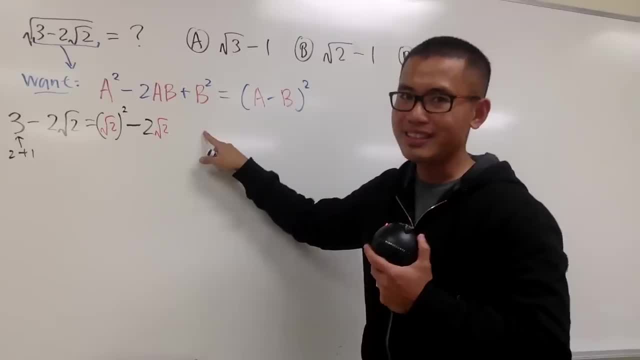 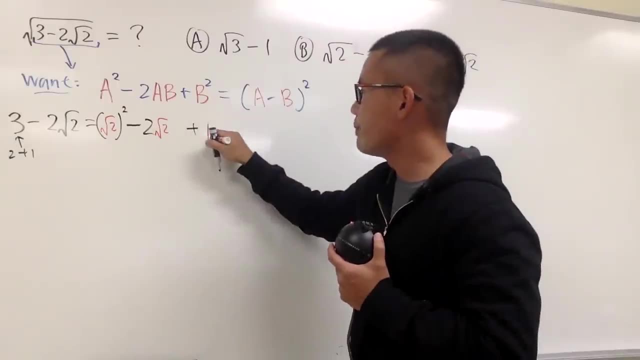 And then this 1 will be going all the way to the end, isn't it? So let me write this down: We have the plus And for 1, let me just put it down right here, And luckily right here- 1 is the same as 1 squared, isn't it? 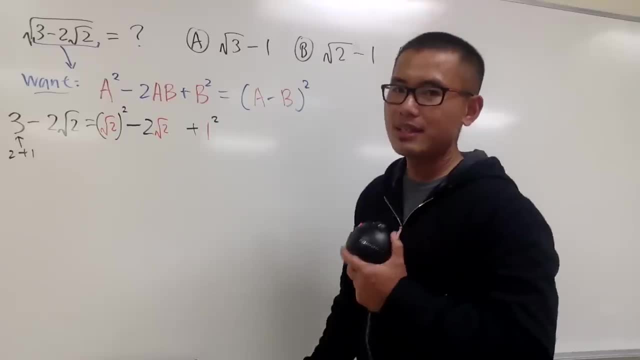 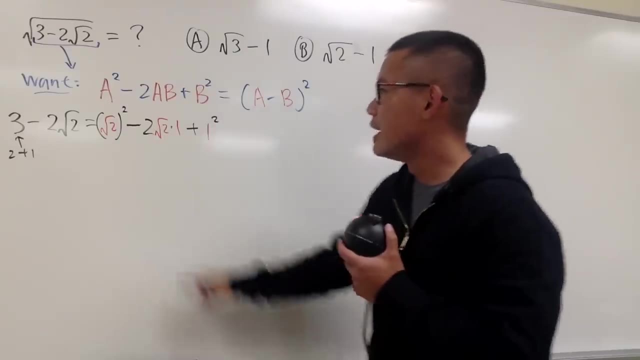 In another word, 1 is the b value, isn't it? And if you would like, you can go ahead and put down times 1.. Of course, you wouldn't change anything when you multiply by 1.. So, as you can see, a is square root of 2, a is square root of 2, b is 1, b is 1..